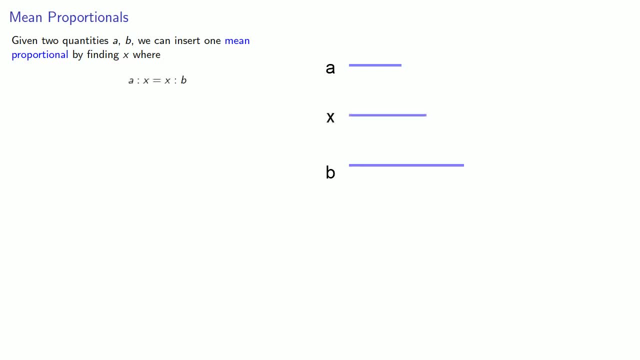 proportional by finding an x where a is to x. And you can see here that in this context, the idea of a mean proportional is that it's some place in the middle, It's some place between a and b. Well, the standard rule in 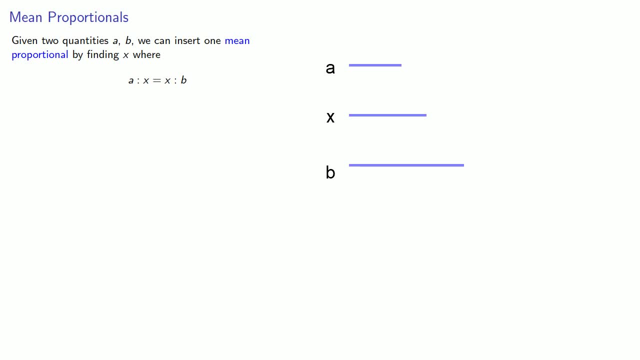 math is anything you can do once. you can do as many times as you want to. So we've put one mean proportional between a and b. Well, let's see if we can insert two mean proportionals, And we'll do that by. 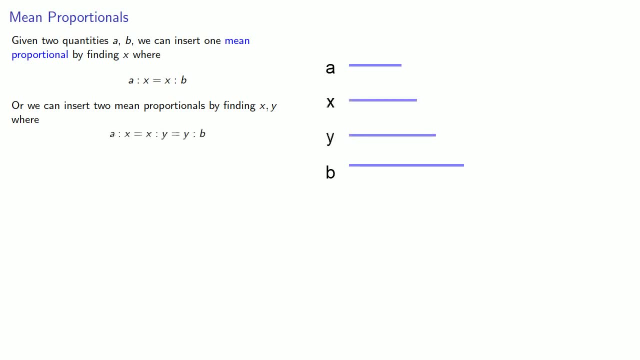 finding x and y, where a is to x, as x is to y, as y is to b, And we can find three mean proportionals: x, y and z, and so on. So another term that will show up is the geometric mean, and that comes from inserting one mean. 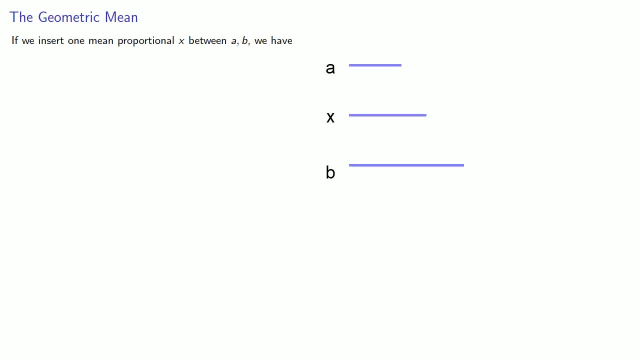 proportional. So if we insert one, mean proportional x between a and b. we have a as to x and we have a as to x, as x is to b, And in modern terms this gives us a over x, is x over b or 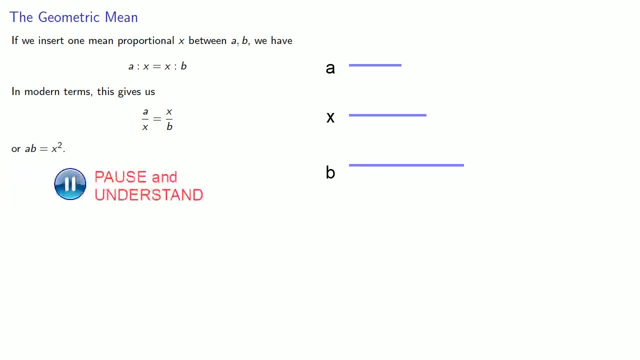 cross-multiplying ab is equal to x squared. Consequently, we have the following result: Given a and b, the mean proportional x satisfies. x is the square root of a times b And x is also known as the geometric mean. So we can: 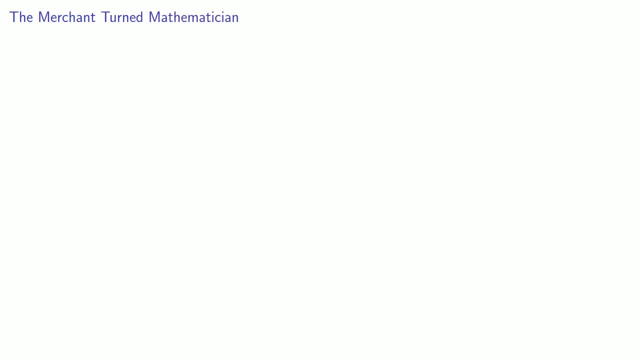 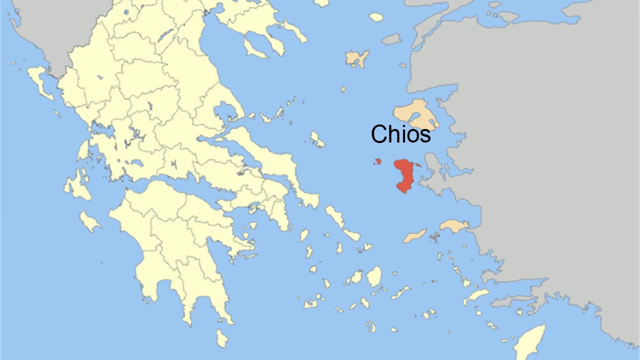 see that x is equal to x over b, or cross-multiplying ab is equal to x over b, or cross-multiplying ab is equal to x over b. So this brings us to Hippocrates of Chios. Chios is one of the many islands that make up Greece, and Hippocrates of Chios shouldn't. 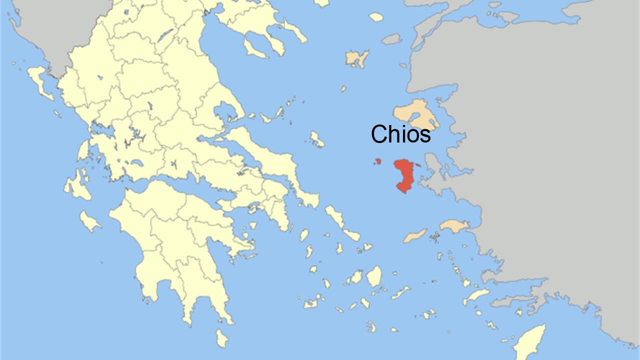 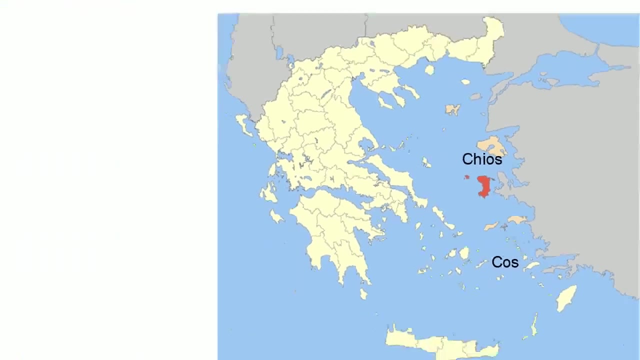 be confused with a much more famous contemporary Hippocrates of Kos. Hippocrates of Kos was the physician. Hippocrates of Chios was the mathematician. We actually know quite a bit about the life of Hippocrates. He lived around 430 BC and. 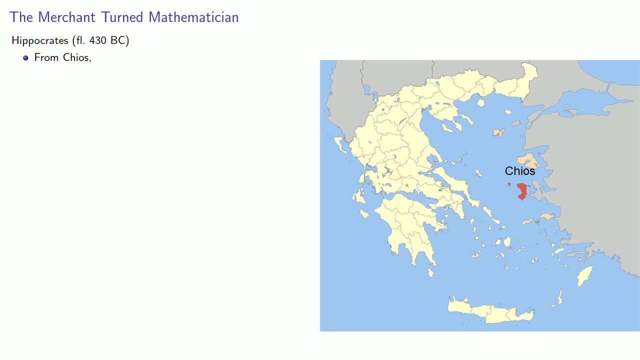 he was a merchant. According to one story, one of his ships was seized by pirates, and he found out that its goods appeared in Athens, and so he went to Athens to try and retrieve them. This required dealing with the Athenian legal system, which took time. So, to keep himself entertained, 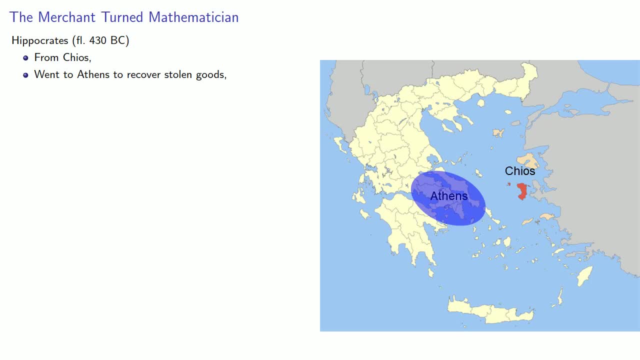 he attended some lectures in mathematics, and after a while he said to himself: Hippocrates, you can do that. And so he became the first person we know by name to be paid to be a teacher of mathematics. Hippocrates also wrote the first known textbook on geometry, which he called the 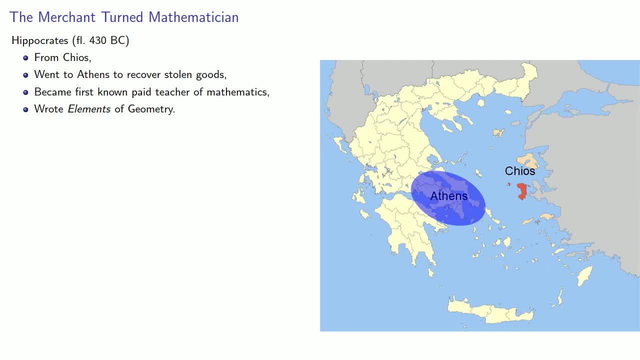 elements. We'll talk about that more later. Now. Hippocrates considered the problem of finding two mean proportionals between a and b, and his results are most easily understood if we rewrite this in a somewhat modernized format. So this first proportionality, a is to x as x is to y, we can. 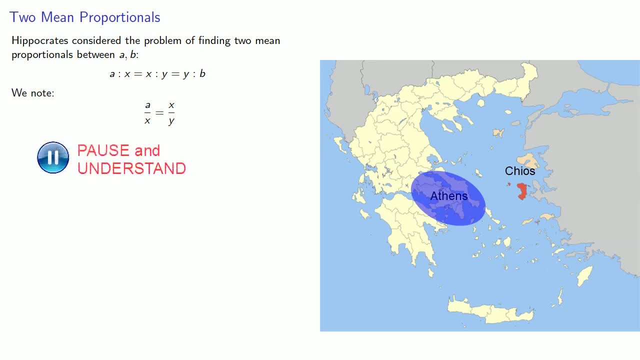 write that as a over x equals x over y, and if we multiply both of these by a over x and simplify, a squared is to x, squared as a is to y. But wait, there's more. If we look at the first and third ratios, that says that a over x is equal to y over b. So this means we can multiply one side by y over. 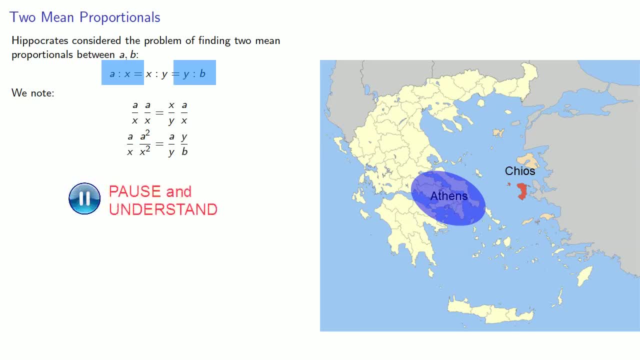 b and the other side by a over x, Then simplify- And this is a very interesting and important result, because if b is to a, then a cubed is to x cubed, as one is to two. But this is exactly what we need to do in order to duplicate the cube. 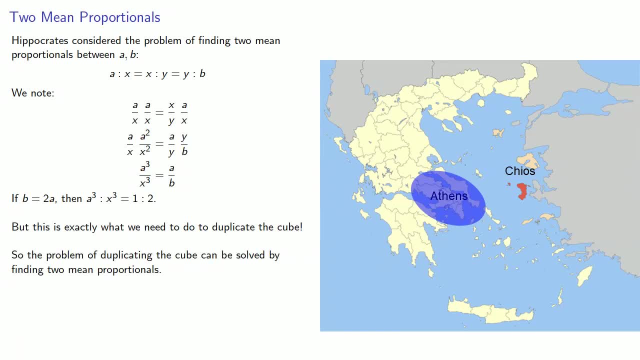 And what that means is the problem of duplicating the cube can be solved by finding two mean proportionals, And it's worth pointing out that Hippocrates didn't know how to do it. He didn't studied a very mathematician thing. He took one problem- duplicating the cube- and it said its the same. 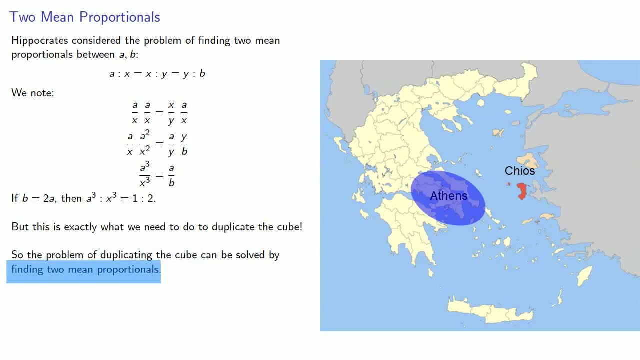 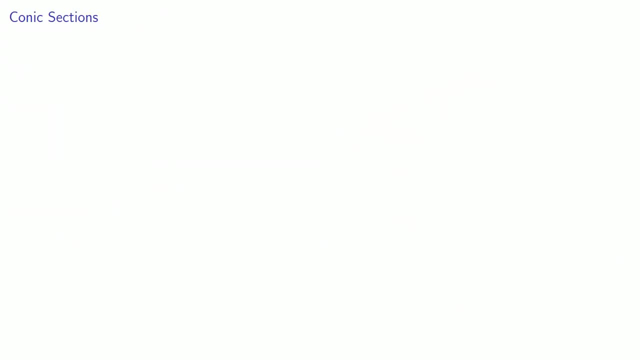 as another problem inserting two mean proportionals. Of course he didn't have any idea on how to solve this problem- inserting two mean proportionals- but it did offer two methods of attack on the same problem And in fact it led to one of the solutions. So, a little while later, Monachemus, living around 350 BC. 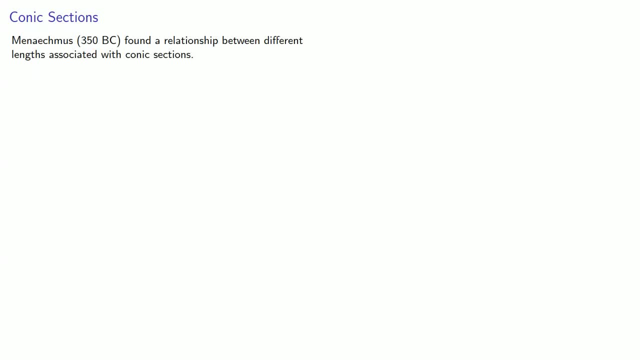 temluesti으 found a relationship between different lengths associated with what we now call conic sections. We'll talk about monogamous work with conic sections elsewhere, but in modern terms we might describe monogamousness results as follows: 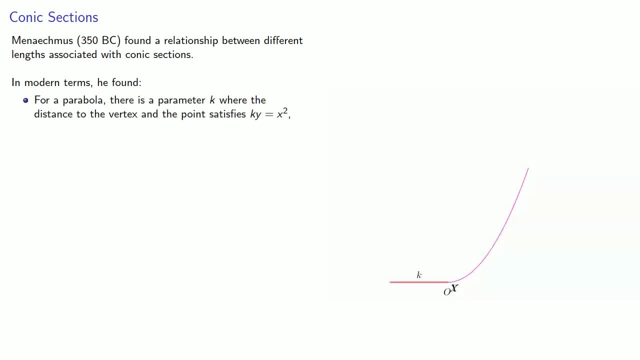 For a parabola, there is a parameter k, where the distance to the vertex and the point satisfies the relationship. ky equals x squared And we might view that as the equality of a rectangle with k and height, y with the square, with the side of x. 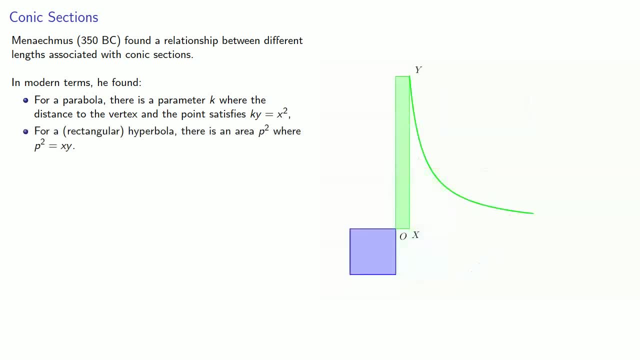 And for what we call a rectangular hyperbola, there is an area p squared, where p squared is equal to xy. Equivalently, the area of a rectangle with one vertex on the hyperbola is equal to a particular square, And monogamous was able to use these relationships. 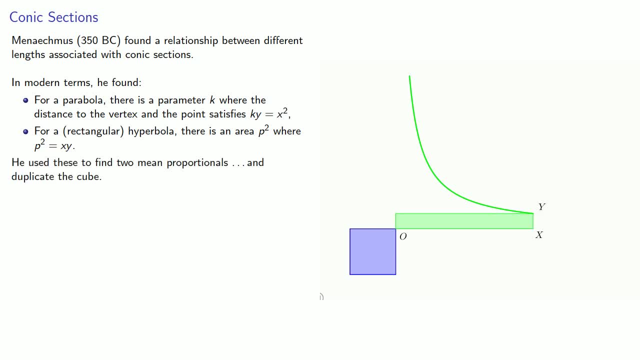 to find two mean proportionals, and because it was the same problem to duplicate the cube. So later Greek writers described a general strategy for solving problems in geometry, analysis and synthesis. In analysis we assume the problem already solved, then try to work towards a starting point. 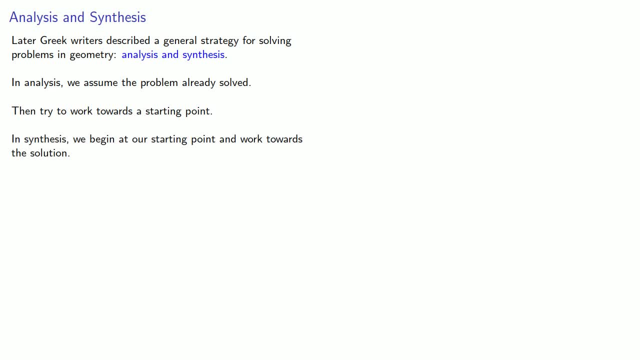 Then in synthesis, we begin at our starting point and work towards the solution. So in this case, suppose we've already solved the problem and we've already found those two mean proportionals, x and y. So we already know a is to x, as x is to y, as y is to b. 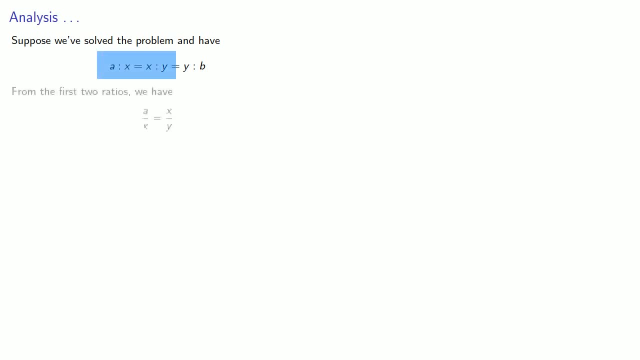 Now, if we take a look at these first two ratios, that gives us a over x, is x over y, And if we cross-multiply, we find that ay equals x squared, which tells us the solutions x and y are going to be the ordnance of a parabola. 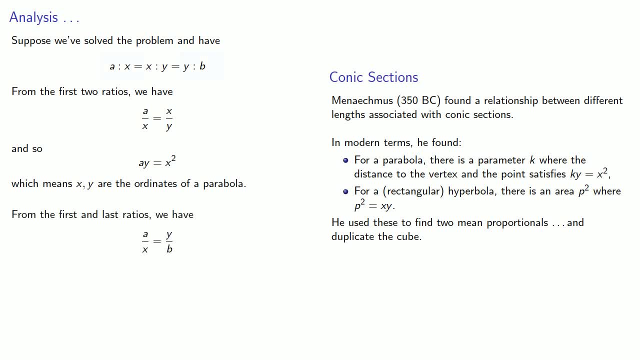 But wait, there's more. If we take a look at the first and last ratios, we have: a over x equals y over b, and cross-multiplying gives us ab equal to xy, which means that xy are the ordnance of a hyperbola.